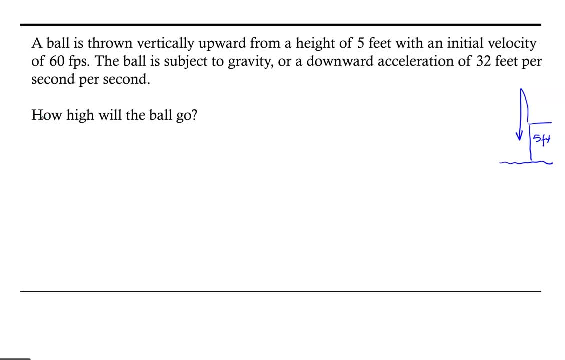 and we want to know, basically, how high this ball goes under these circumstances. Now, what do we know in this problem? First of all, we know that we have the ball starting from a height of 5 feet, so we know that the initial position of the ball 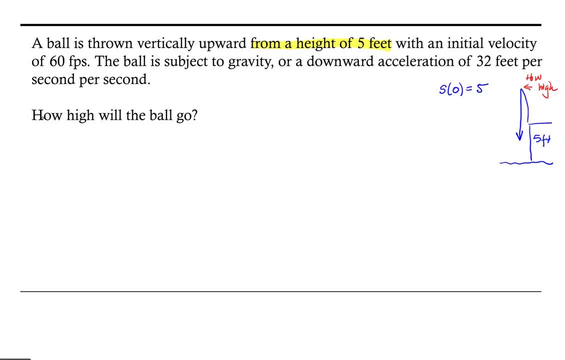 when it's thrown is 5 feet. What else do we know? We know that the ball is thrown with an initial velocity of 60 feet per second. So we know that the velocity at time zero is 60 feet per second. We also know that the ball is subject to gravity or a downward acceleration of 32 feet per 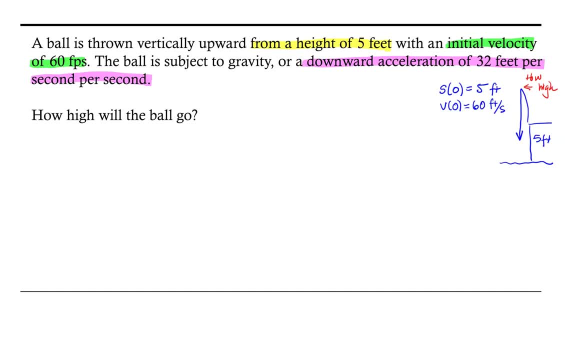 second per second. So we know that there is this downward acceleration that is, 32 feet per second per second. This mean and it's downward, so this would be negative. So with this information we should be able to get started. Now what do we know about acceleration? 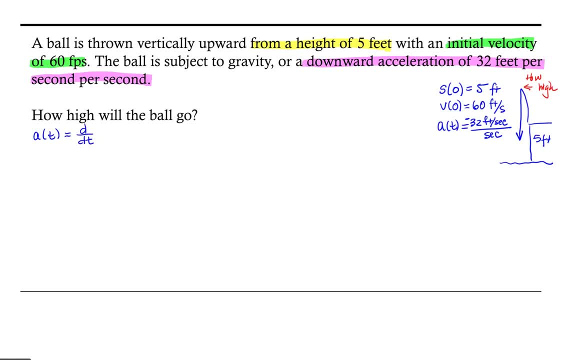 We know that acceleration is the derivative with respect to time of velocity. So what that tells us is that velocity should be the antiderivative of velocity, The antiderivative of acceleration. And if that's the case, then in this particular instance, the velocity is the antiderivative. 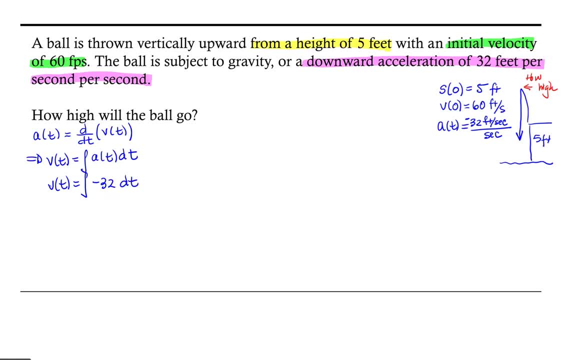 of negative 32 dt, Which is the same as negative 32 times 1 dt, Which would be negative 32 times t, T being the antiderivative of velocity Of 1 dt plus our constant of integration. Now, what do we know about velocity? 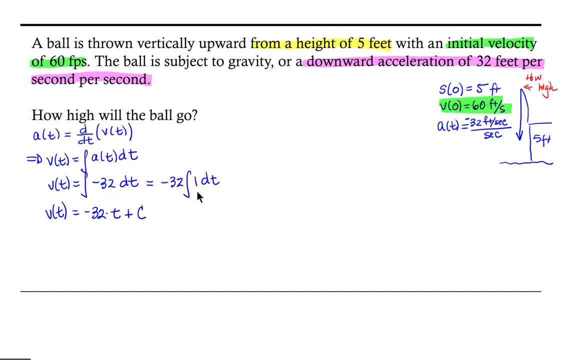 We know that velocity at time zero is supposed to be 60 feet per second. So what that tells me here is that in this case, for this velocity function, that negative 32 times t is the antiderivative of velocity. Negative 32 times 0 plus c should equal 60. 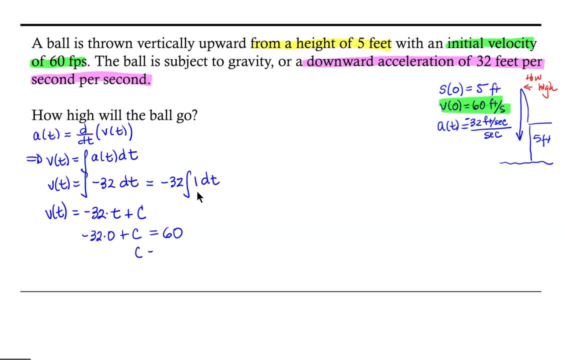 Negative 32 times 0 is 0.. So c should equal 60.. Which means then that our velocity function for this instance or this occasion, is negative 32t plus 60.. So there's our velocity function. Now, what do we know about velocity? 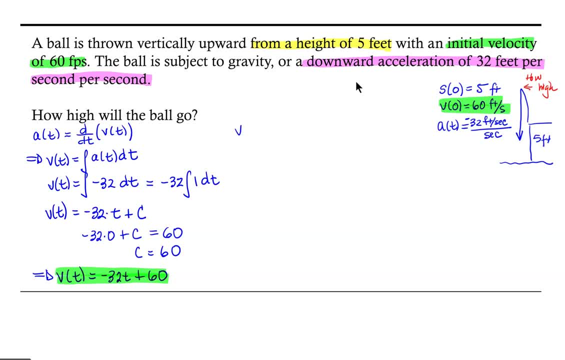 Well, we know that velocity v of t is the derivative of position. So that should mean that position is the antiderivative of velocity 0.5.. 0.5. And in this particular case, position should be the antiderivative of negative 32T plus 60DT. 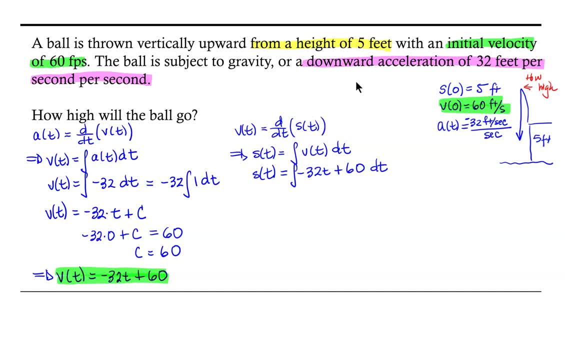 So if we integrate this, we get: S of T is equal to negative 32 times the antiderivative of TDT, plus 60 times the antiderivative of 1DT. So S of T is equal to negative 32.. The antiderivative of 1DT is equal to negative 32.. 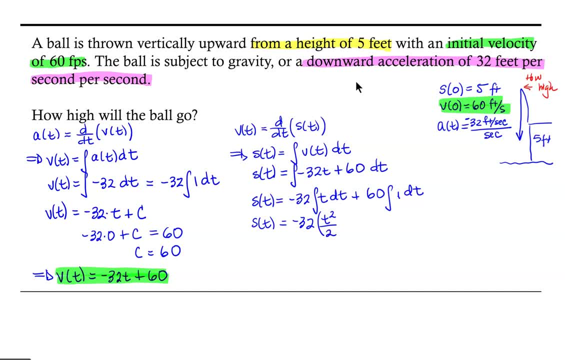 So S of T is T squared over 2 plus 60 times the antiderivative of 1 is T. And then we do have our constant of integration C. So S of T- simplifying here a little bit- is negative 16T squared. 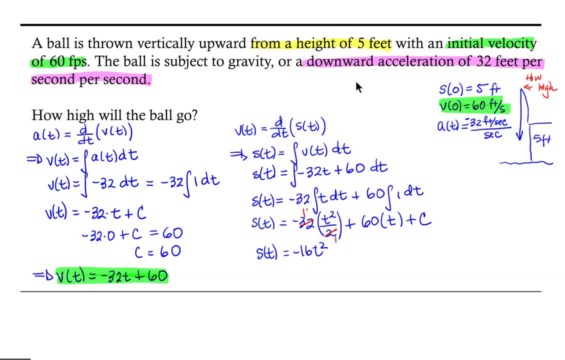 2 will divide into 32.. 16. Times Plus 60T plus C. And now we know that the ball was thrown from a height of 5 feet. So we know that initially the position is 5 feet. So using that information in our position function here when T equals 0,. 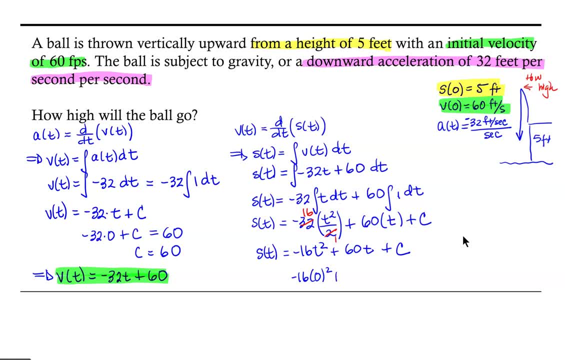 we get negative 16 times 0 squared, plus 60 times 0 plus C, And that's supposed to equal 5.. Well, 16 times 0 squared is 0.. 60 times 0 is 0.. So we have 0 plus 0 plus C is equal to 5.. 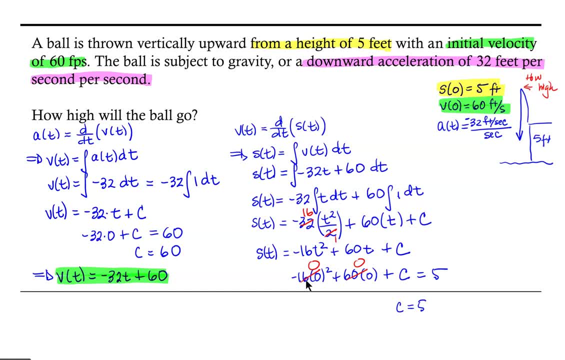 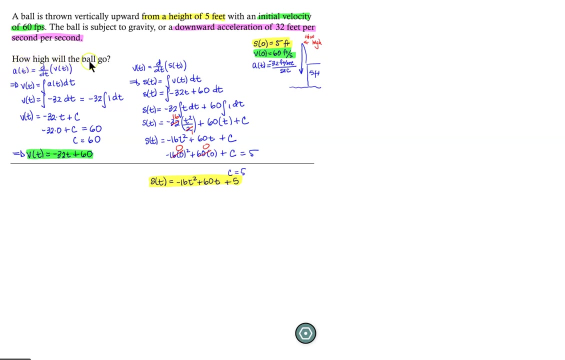 So this tells us that C should equal 5.. And overall, then, this tells us that our position function should be negative: 16T squared plus 60T plus 5.. So recall that our task here was to figure out how high the ball will go. 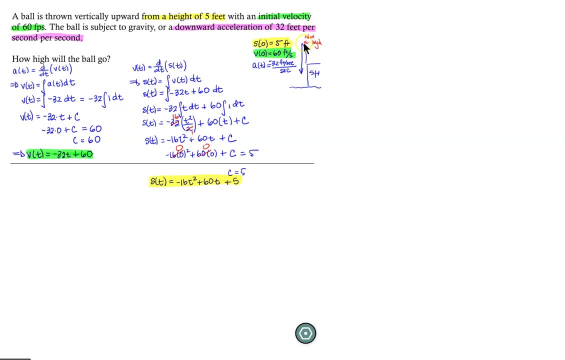 So if we look at this drawing, what we want to know is this height: How high will the ball go After it's thrown? So what we're looking for is the maximum position or the maximum height of the ball, So describing this in calculus terms. 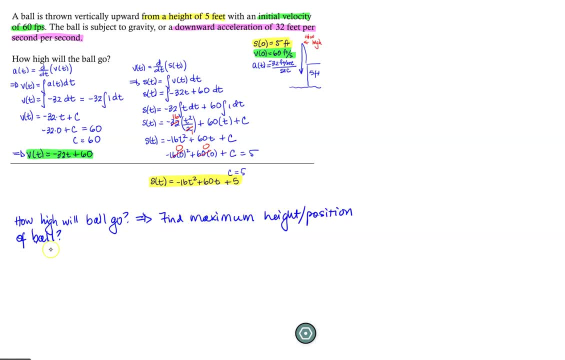 what we're interested in is finding the maximum height or position of the ball. So we have our position function, And how do we find the maximum of that function? Well, we find the critical points of its derivative. And what is the derivative of our position function? 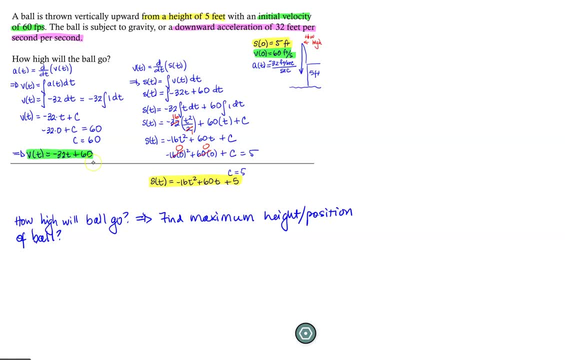 Well, the derivative of our position function is the velocity function, And we do have that. So what we want to do is find the critical points of the derivative of position That also happens to be the velocity function, And the critical points come from two places. 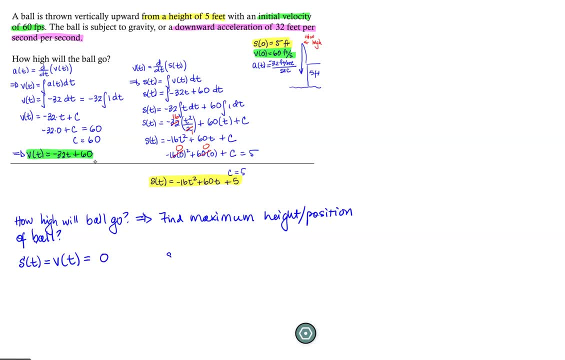 Where that derivative equals 0. And that derivative equals 0. And where that derivative is undefined. Now notice that our velocity function, our derivative, is a nice linear function, So we won't be finding any critical points where the derivative is undefined. 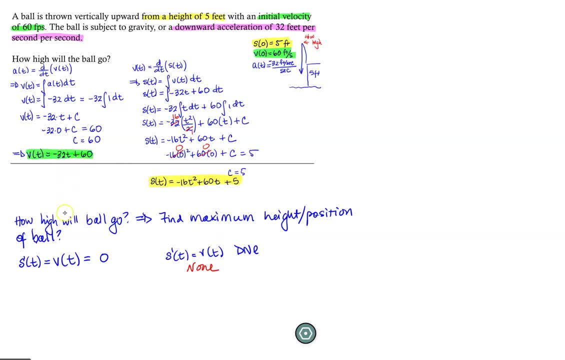 because it's defined for all real numbers. So we're left looking for critical points by setting the derivative equal to 0. So we get negative 32t plus 60 equals 0. If we add 32t to both sides of the equation, we get 60 equals 32t. 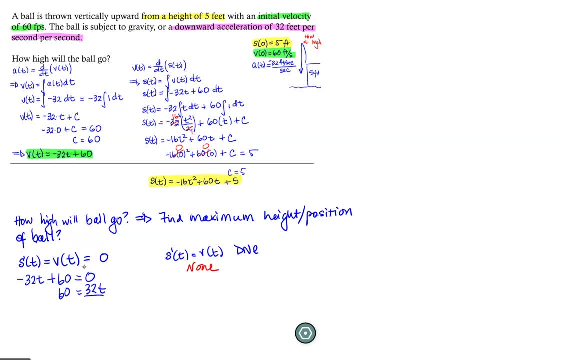 And then if we divide both sides of this equation by 32, we get that t is equal to 60 over 32.. Now 4 goes into both 60 and 32.. 4 goes into 60 15 times and 4 goes into 32 8 times. 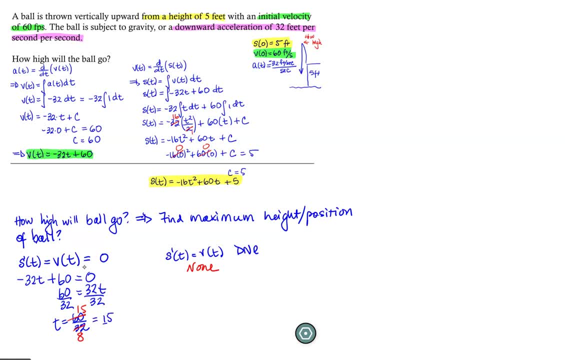 So our t is 15 over 8, and that can actually be written as a terminating decimal. That is 1.875 seconds, So that's the time at which the derivative of our position function equals 0. And we anticipate that being a maximum. 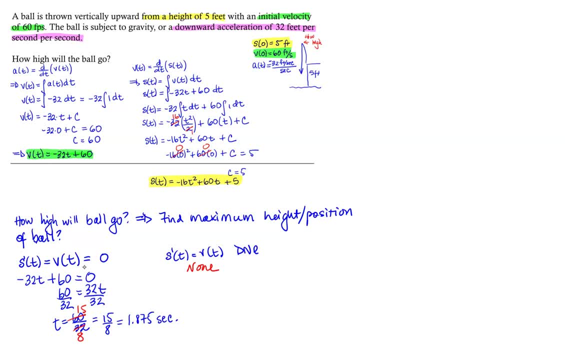 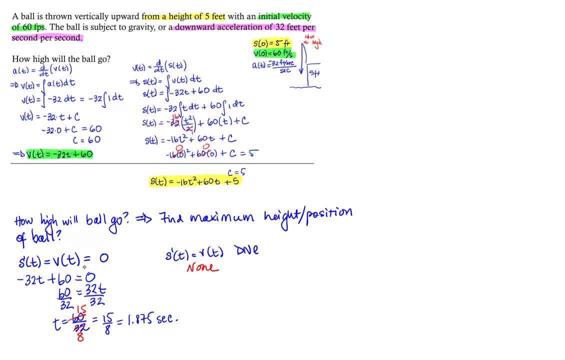 I'm going to use the second. I'm going to use the second derivative test because it's easy to use and I actually have the second derivative already available. The first derivative of position was velocity. The second derivative of position is acceleration And our acceleration function, we saw, was negative 32..